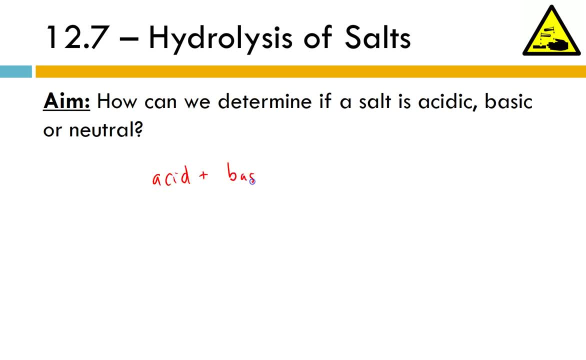 we've been talking about this reaction. An acid plus a base produces salt plus water And so far the salt hasn't really been getting too much attention. We've looked at the strengths of the acids and bases. We know that we produce water as the actual neutralization between the H. 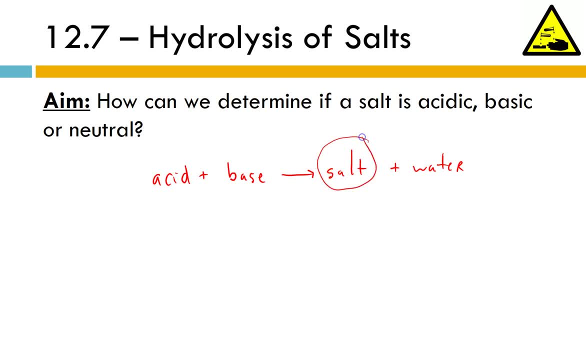 plus and the OH minus. But it turns out the salt is actually pretty important too. Now, the salt based on how it was formed, in other words, which acid and base were used to neutralize each other, can be acidic, basic or neutral itself. So I could take this salt, I could dissolve it in water. 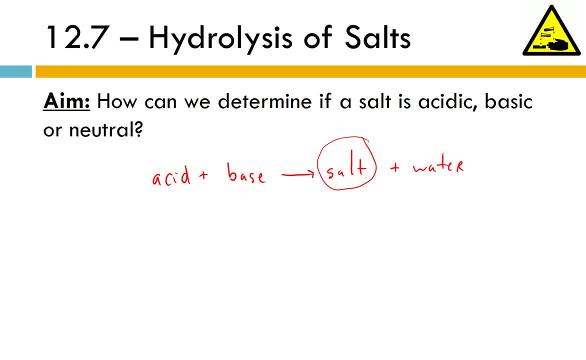 and when I measure the pH, the pH might actually be not neutral. It could be acidic or basic. So it's kind of weird. It's weird to think about a salt that doesn't have any H plus or OH minus ions present in it. 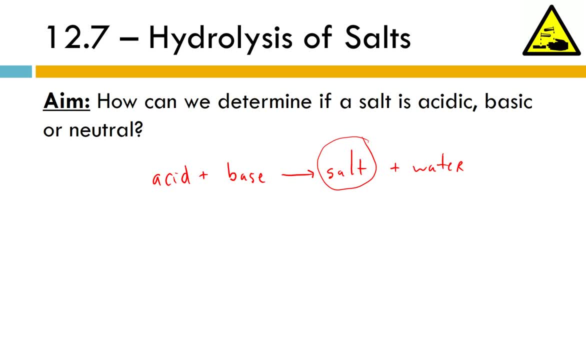 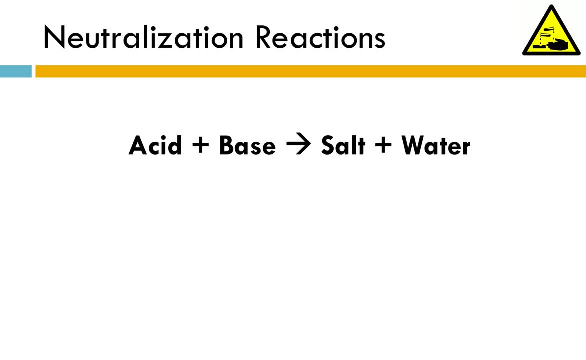 impacting the pH, But that does in fact happen and we're going to talk about it today. All right, hopefully you are so sick of seeing this equation by now. Acid plus base yields, salt plus water- a very specific type of neutralization And, sorry, a very specific type of double. 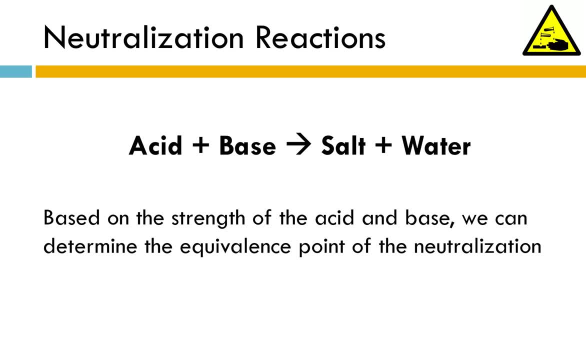 replacement. I should say Based on the strength of the acid in the base, we can determine the equivalence point of the neutralization. That's what we talked about in the previous lesson. If you have a strong acid and a strong base neutralizing each other, you get a neutral. 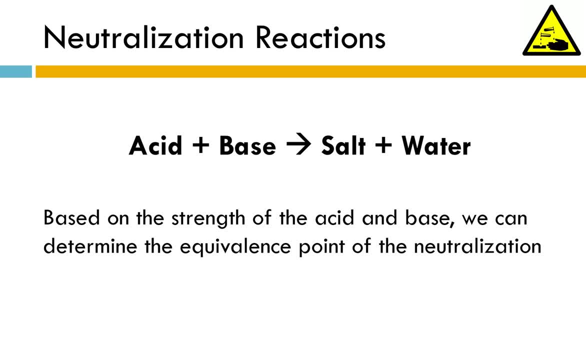 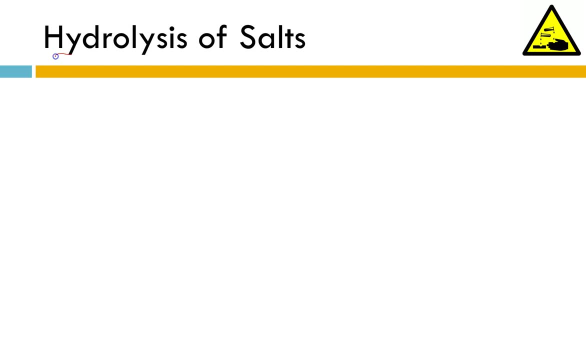 equivalence point: strong acid- weak base. acidic equivalence point: weak acid- strong base, a basic equivalence point and we don't ever really titrate weak acid plus weak base. So when it comes to hydrolysis of salts- hopefully with the word hydrolysis you see hydro built- 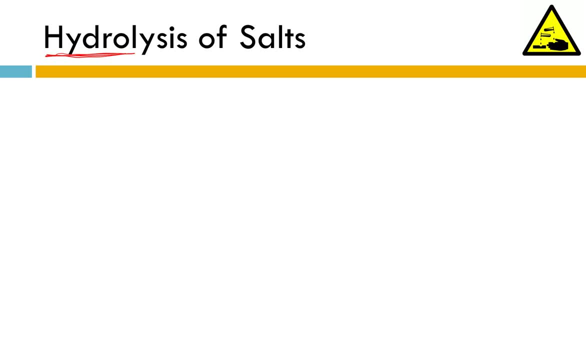 right into the front, and that's talking about water. We're talking about dissolving these salts in water, So, based on the identity of the salt, we can work backwards to try to determine what acid and base were reacted. We know that the cation is always going to come from the base. Think. 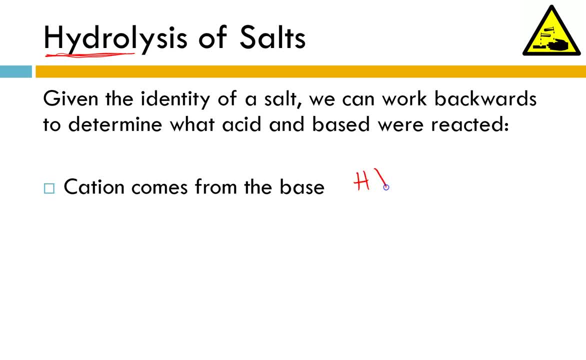 about it. Our acids are always HX, X just being some anion. So the cation from an acid is always a hydrogen ion. The anion is going to come from the base We always have. we'll use Y, not for yttrium. You know that's probably not a good idea. Let's do. 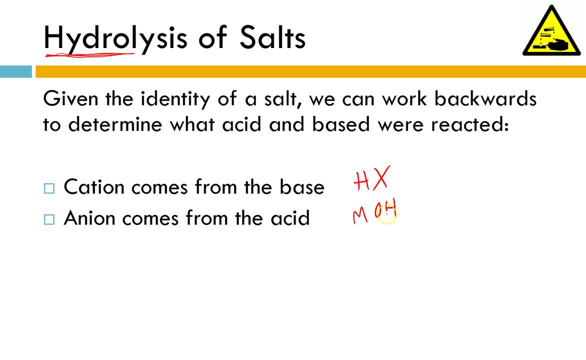 M for metal. The anion for a base is always going to be hydroxide, So the anion must come from the acid And then, based on the strength of the acid in the base that were used to produce that salt, we can determine if the salt is acidic, basic or neutral. So let's go through and do an example. 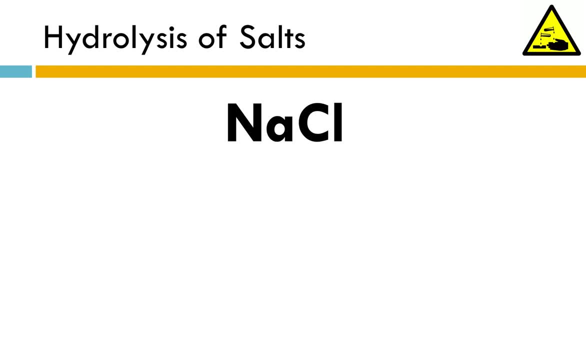 Let's talk about NaCl, sodium chloride, something you're very familiar with. We know that the cation has to come from the base, So this had to be a base. So we're going to look at sodium hydroxide. We're only going to look at Arrhenius acids and bases, The chloride. 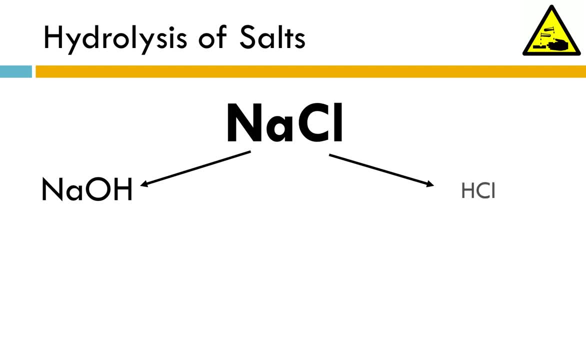 ion must have come from the acid. That means that it came from HCl, hydrochloric acid. Sodium hydroxide is a strong base. Hydrochloric acid is a strong acid. So if I was to take sodium chloride, dissolve it in water and measure the pH, I would see that the pH is equal to 7. It's neutral. 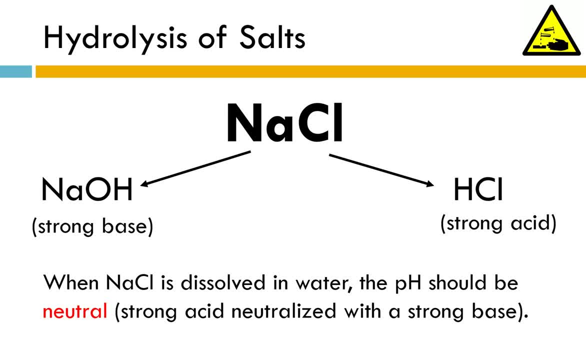 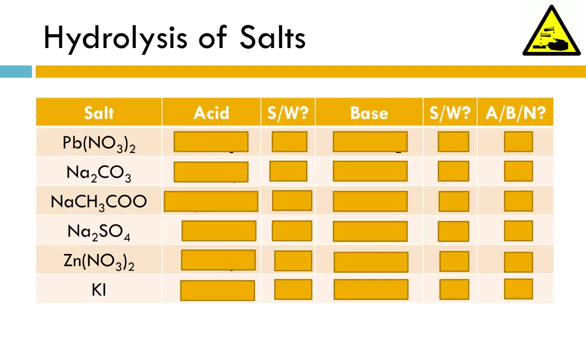 Sodium chloride is a strong base. Sodium hydroxide is a strong base. Sodium hydroxide is a strong base. Sodium hydroxide is the product of a strong acid and a strong base. So we have a neutral or relatively neutral salt. Let's try some practice problems In class. we'll actually go through and 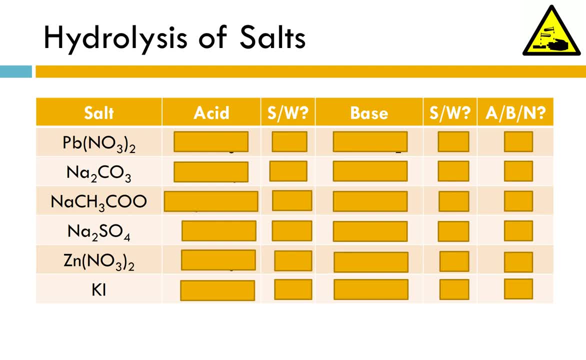 test the pHs. Needless to say, that's going to be hard on a PowerPoint slide, So we'll just do a little bit of practice. We've got the salt. I want you to give me the formula of the acid and the base, Tell me if that's a strong or weak acid and base and then predict the endpoints. So I'll go. 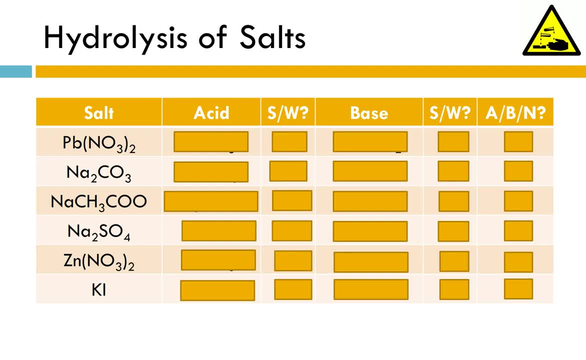 in with you just to make sure you've got the hang of it. All right, we have PbNO3-2, lead to nitrate, So we know the cation comes from the base. So that must have been PbOH in parentheses 2.. 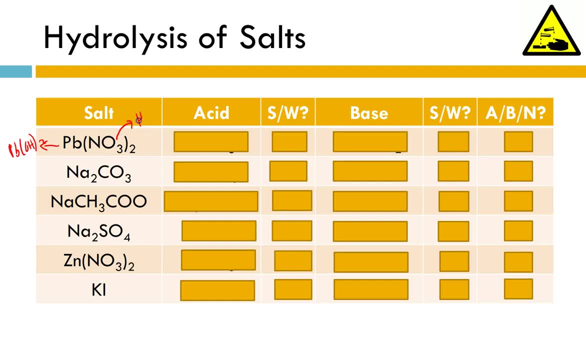 And we know that the anion comes from the acid, So this is probably HNO3.. So let's check. Yeah, HNO3.. Nitric acid: is it strong or weak? Now this is a strong acid, No way to tell, just by. 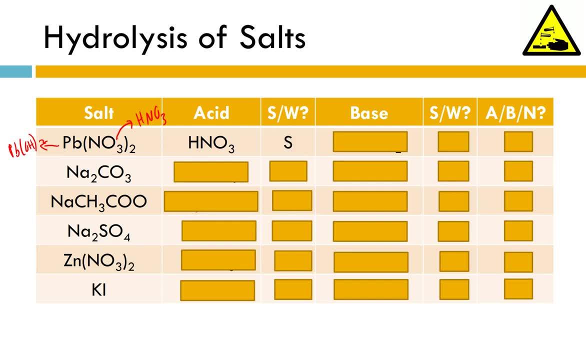 looking at it, You have to memorize your seven strong acids. So let's go ahead and do that. Let's check our base Lead 2-hydroxide. Good, we got it right. Strong or weak? Yeah, this isn't on. 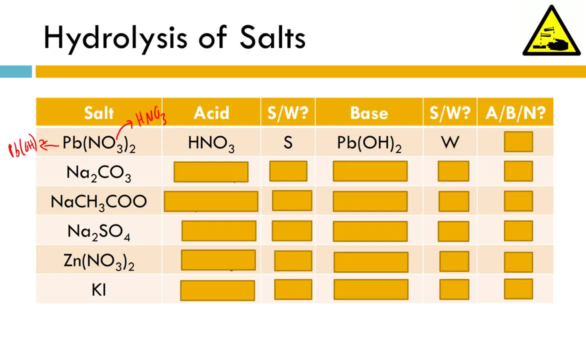 our list of seven strong acids. This is a weak base. So if we have the salt, a strong acid plus a weak base, we will see an acidic endpoint. Go ahead, pause the video and try out the remaining five questions. We'll review them together. 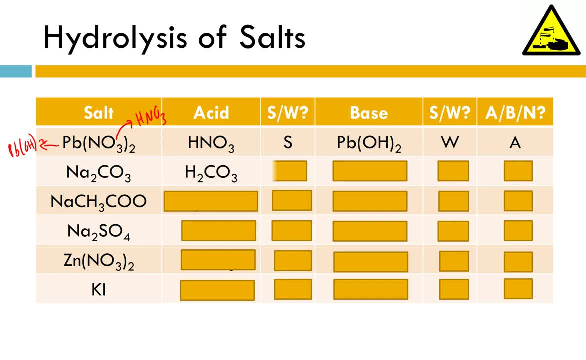 All right, we've got sodium carbonate- That's coming from carbonic acid, a weak acid- and sodium hydroxide, which is a strong base. So strong base plus weak acid, that's going to give us a salt that is basic in nature. So when I 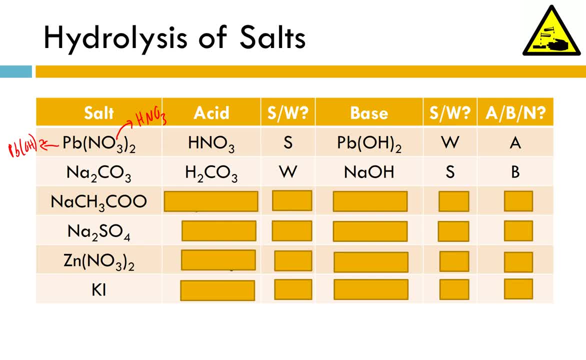 dissolve sodium carbonate in water and I test its pH. it's going to be above 7.. Up next we have sodium acetate. Acetic acid is our acid. That's the active ingredient in vinegar. It's a weak acid. You wouldn't want to ingest strong acids. Our base again is sodium hydroxide, which is a 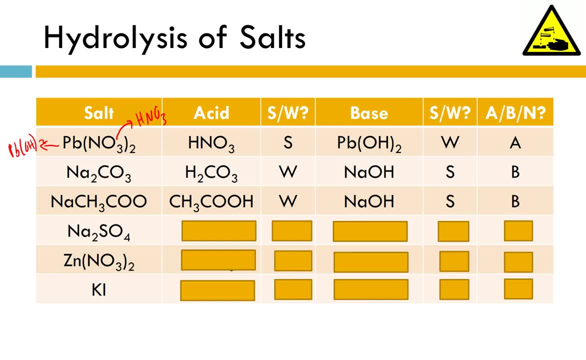 strong base. So we see another basic salt: Sodium sulfate. Sulfuric acid must be the acid That's strong. Sodium hydroxide is our base, Also strong. So strong plus strong gives us a neutral salt. So when that's. 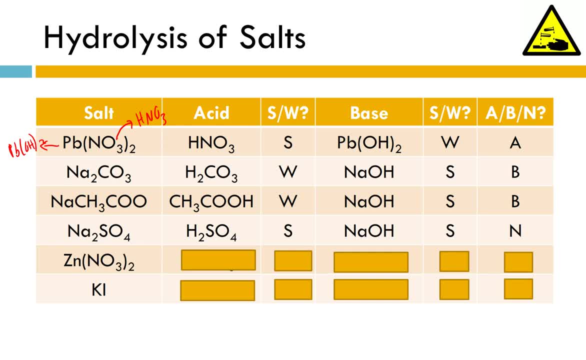 dissolved in water, like sodium chloride, we'll see no real change in pH. Zinc nitrate- HNO3,, nitric acid, strong acid. Zinc hydroxide, a weak base, We'll have an acidic salt. This will cause the pH to drop when it's dissolved in water. And, last but not, 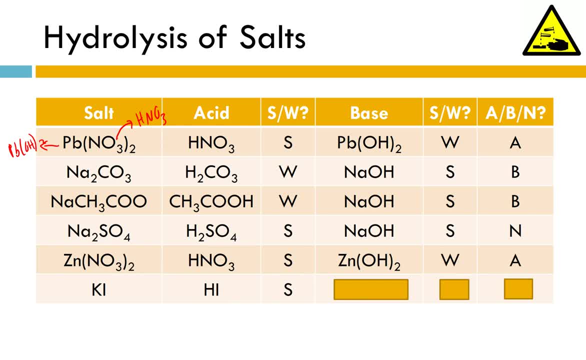 least we have hydroiodic acid- It's one of our seven strong acids- Potassium hydroxide, one of our seven strong bases. So we end up with a neutral salt. All right, that's really the gist of it. 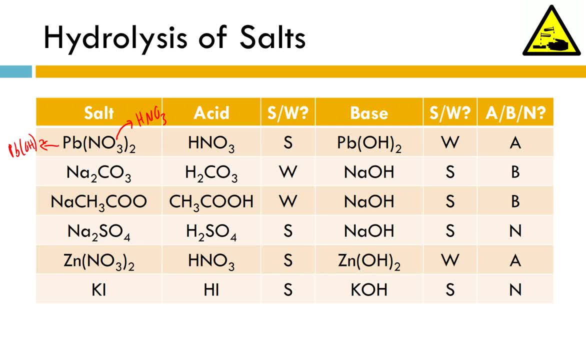 So we're just doing the opposite of all those acid-base neutralization reactions that we talked about the last couple lessons. Instead of trying to predict the formula, we're just trying to predict the formula of the salt. We want to backtrack and we want to know the formula of the acid and the base. 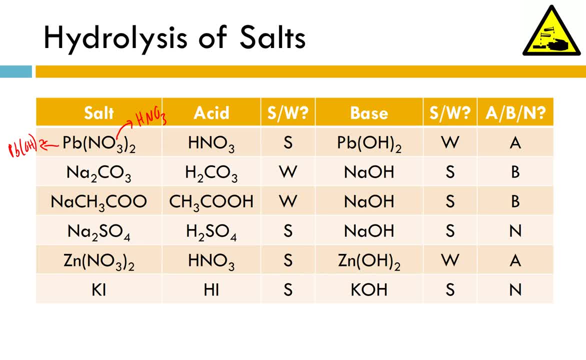 that were used to create that salt. In order to predict whether the salt will be acidic, basic or neutral, you need to know the seven strong acids and seven strong bases. I know I've said it dozens of times by now. I'm so sorry for repeating myself to those of you who have. 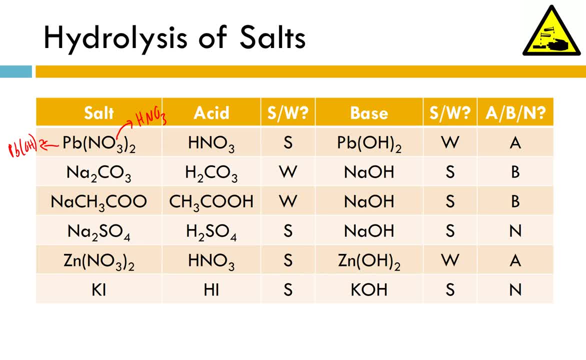 actually gone through and memorized them, but I can assure you not everybody has. You need to know them If you're flipping back and forth to that page to check the strength of an acid or a base. you don't have them memorized and you need to carve out like two minutes over the next couple. 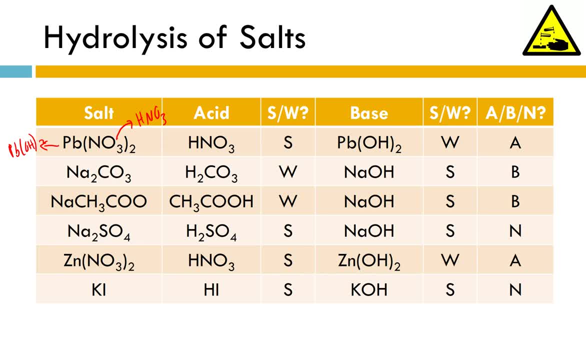 of days to really get those stuck in your head. All right, well, thank you for tuning in. I hope you found this helpful and I'll see you again soon. 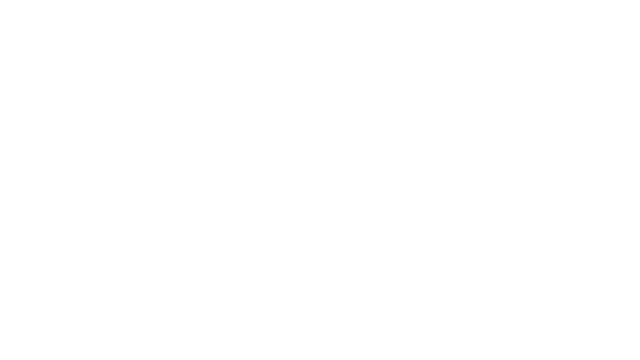 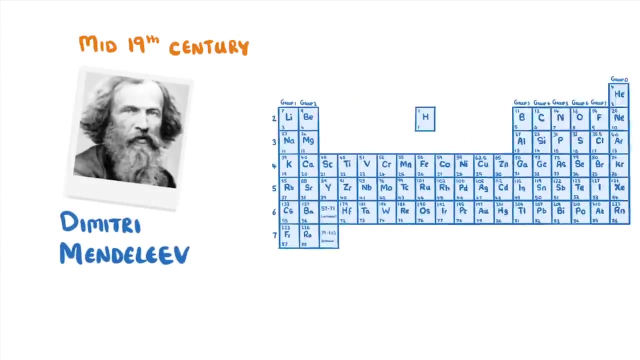 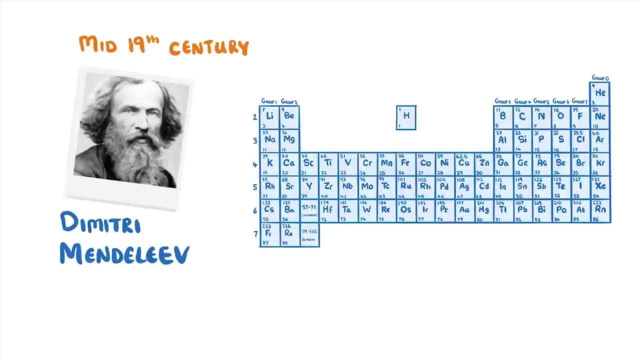 Dimitri Mendeleev was a Russian chemist and inventor, and back in the mid-19th century he devised the periodic table, which organised all of the known elements. In fact, when he made it, it even predicted new elements that we hadn't discovered yet. 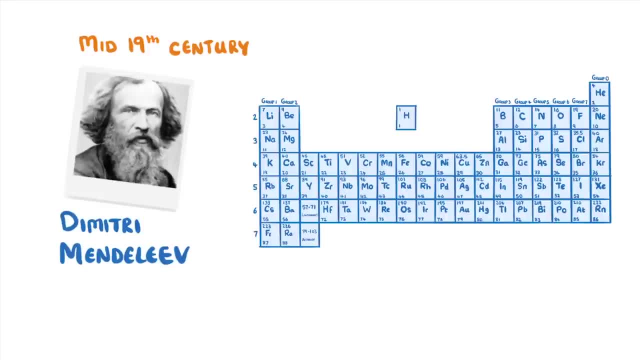 As we saw in our video on elements, everything in the universe is created from different combinations of the elements. in this table, Just like a book, it's read from left to right and from top to bottom, with the elements arranged in order of increasing atomic number. 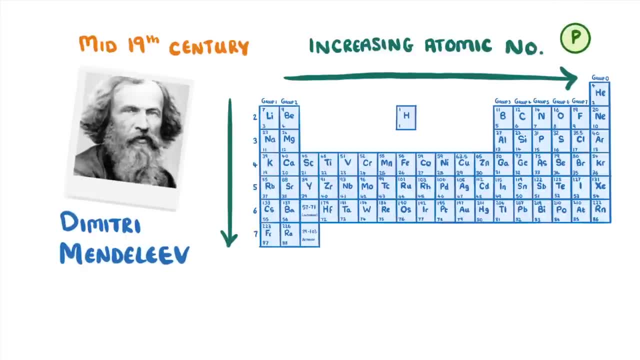 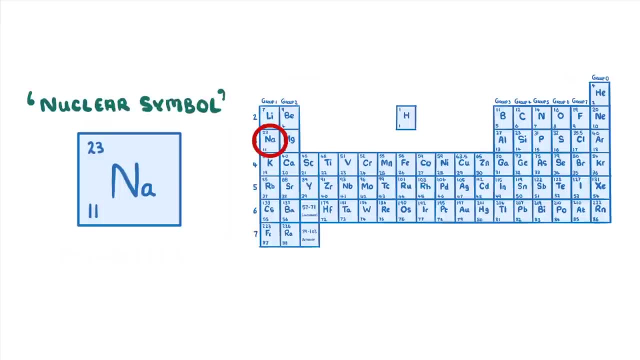 which represents the number of protons in the atoms of that element. Within each of these boxes is the nucleus symbol for that element, which has three components. On the right we have the elemental symbol, which is the one or two letter symbol for that element. 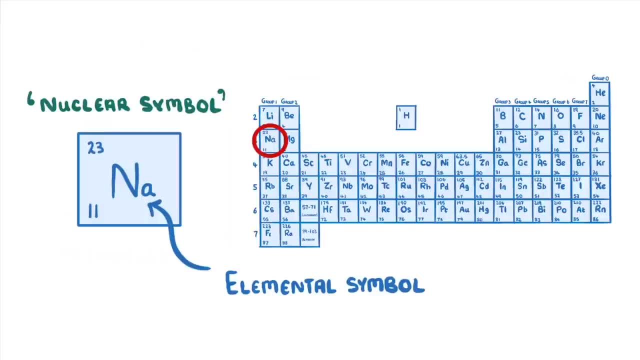 In this case Na, which stands for sodium. In the bottom left we have the atomic number, which tells us how many protons the atoms of that element have, And in the top left we have the mass number, which tells us the total number of protons. 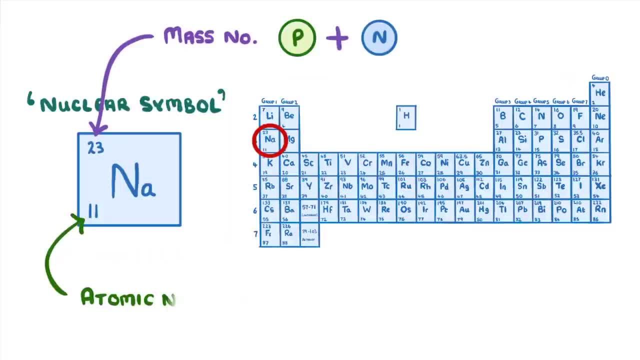 and neutrons in that atom. While he was organising the table, Mendeleev found that the elements displayed a pattern of chemical properties that repeated at regular intervals. So instead of arranging the elements in one wrong line, he formed a new row every time.